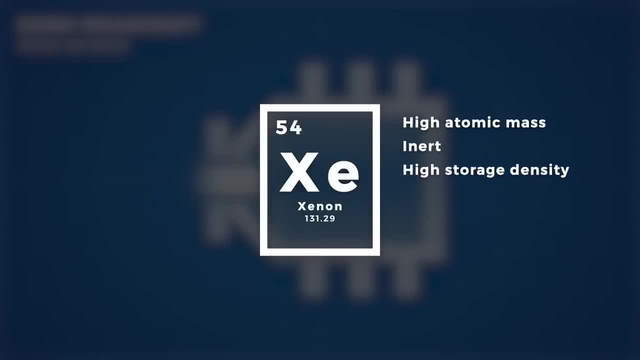 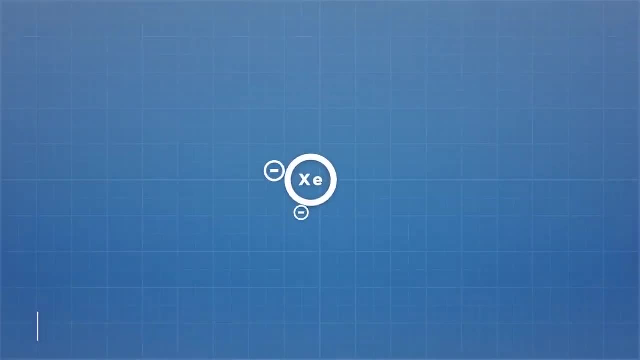 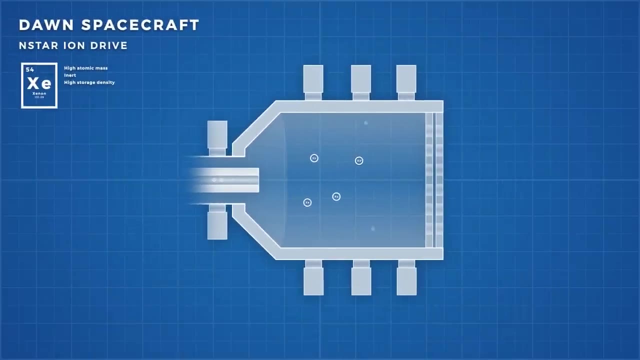 and having a high storage density, lending itself to long term storage on a spacecraft. The engine releases both xenon atoms and high energy electrons into the ionisation chamber, where they collide to produce a positive xenon atom and more electrons. These electrons are then collected by the positively charged chamber walls. 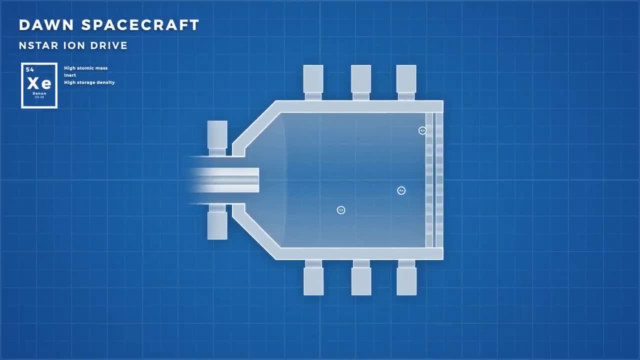 the positive xenon atoms migrate towards the chamber exit, which contains two grids: a positive grid called the screen grid and a negative grid called the accelerator grid. The high electrical potential between these grids causes the positive ions to accelerate and shoot out of the engine at speeds of up to 145,000 kilometres per hour. 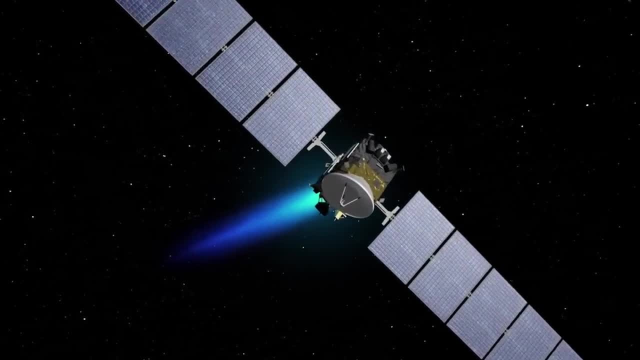 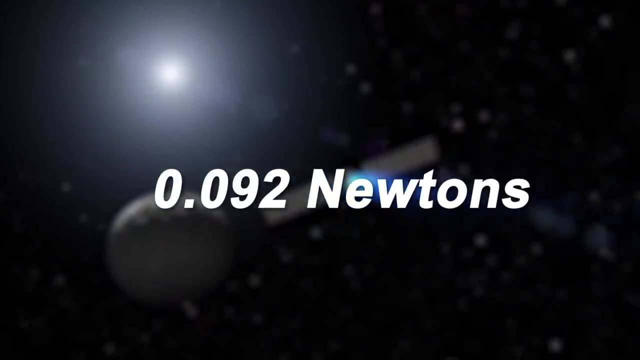 At that speed, even the tiny xenon atoms can provide a decent bit of thrust, but even still, this engine provides a maximum of 92 millinewtons of force- About the same force a piece of paper will exert while resting on your hand. 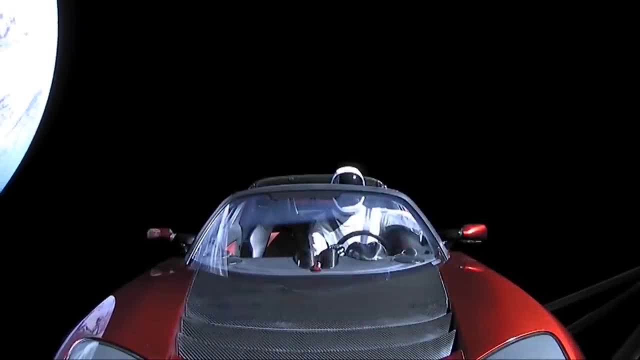 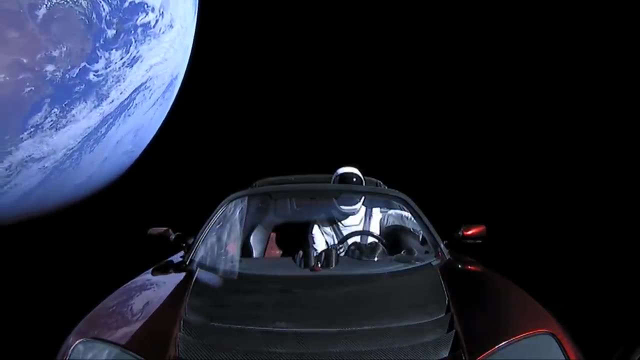 But in the vacuum of space there is no air to sap away the precious energy we provide. with no drag or friction to remove energy, we gradually build our kinetic energy and gain speed. The Dawn spacecraft weighed about 1220 kilograms at launch. 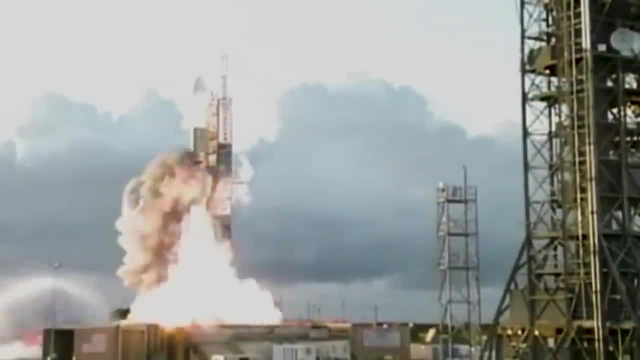 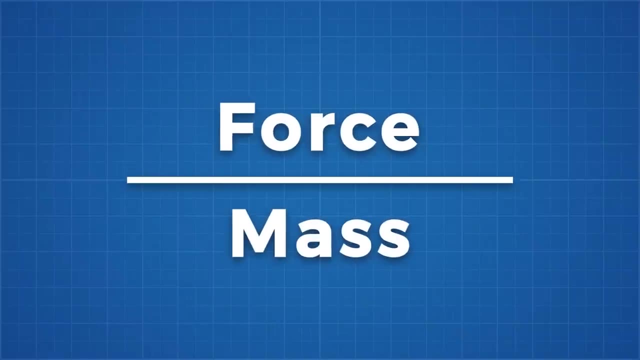 with a dry mass of 750 kilograms after the propellant had been expended. so let's say it has an average weight between the two of 1000 kilograms. Rearranging the force at the top of the spacecraft is a very important step. 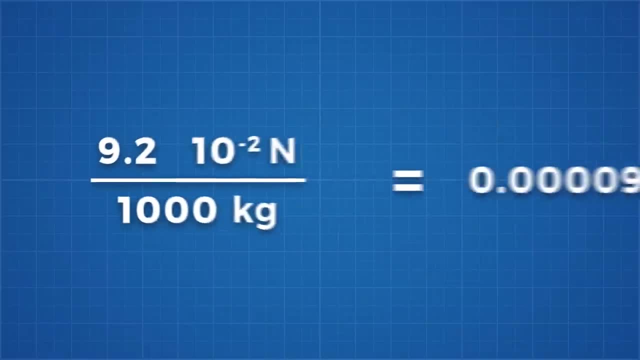 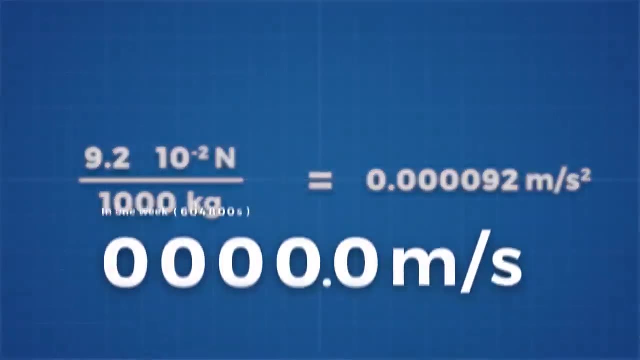 because if the force equals mass, by acceleration equation, we can calculate the acceleration this engine can provide at 0.000092 meters per second. squared, A tiny acceleration, but multiplied by a week and our spacecraft is flying at 55.6 meters per second. 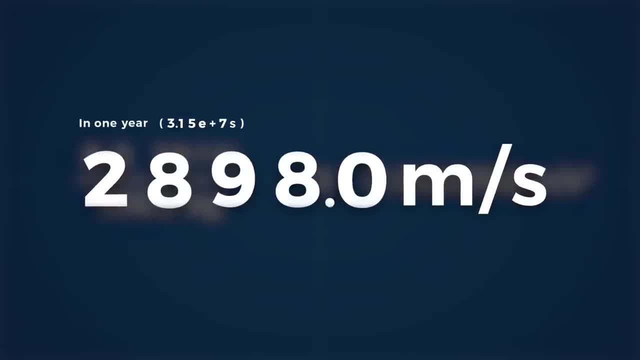 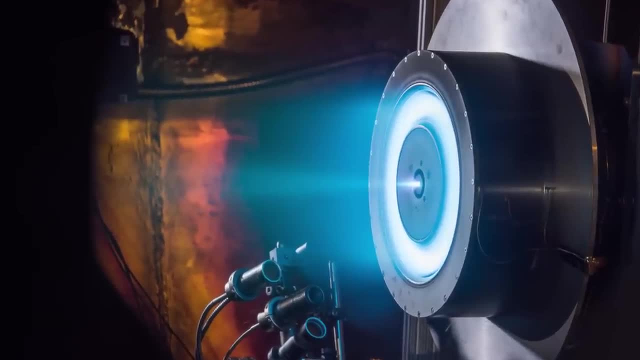 multiplied by a year and it's flying at 2898 meters per second, that's 8.5 Mach. The latest generation ion drives, dubbed the next engine, can produce three times the force and have been tested continuously without stopping for six years straight here on Earth. 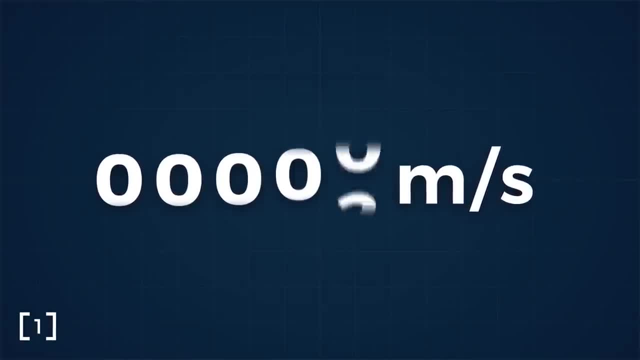 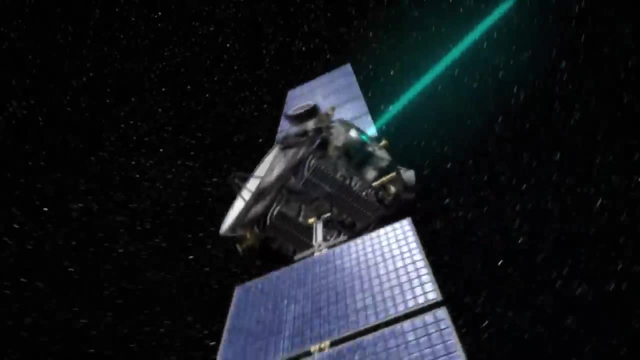 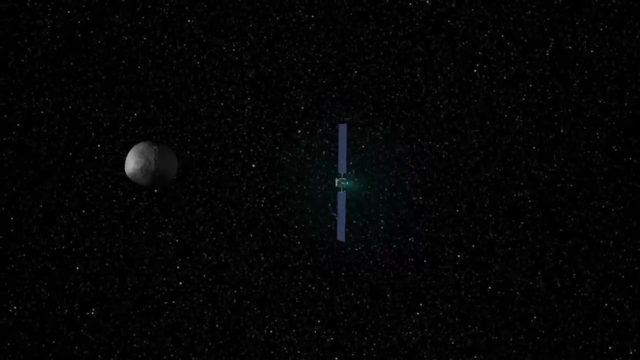 That's enough force to accelerate that 1000 kilograms to 44,651 meters per second, 130 times the speed of sound. This is an incredible technology that will revolutionise how we explore space in the near future. but here on Earth it has a completely different set of challenges. 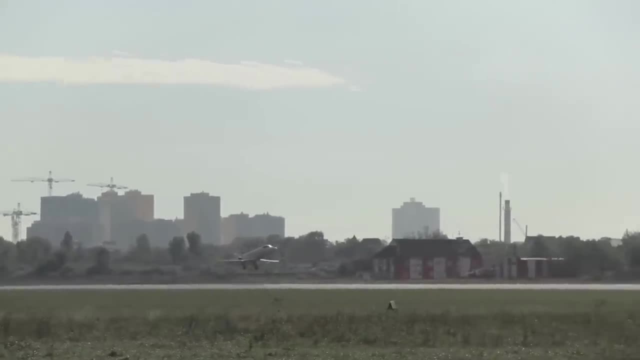 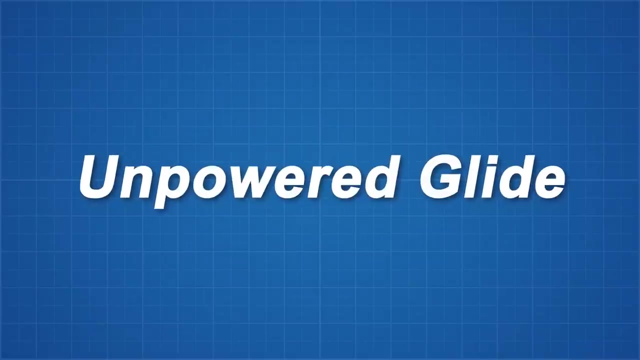 Here on Earth, planes pose a completely different challenge. Air will continuously sap away any energy we input into our environment, and we will be able to use that energy to create more and more energy for the future of our planet. So we need to create an ion drive that can provide more energy than air can remove. 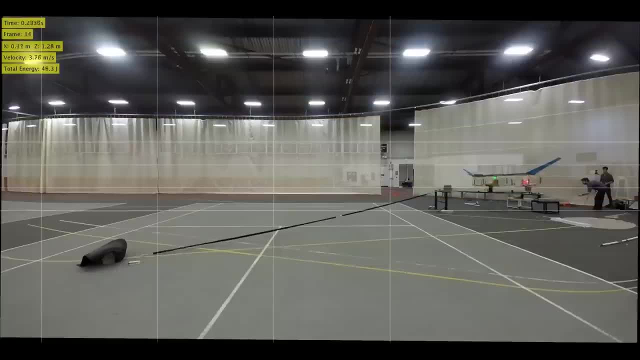 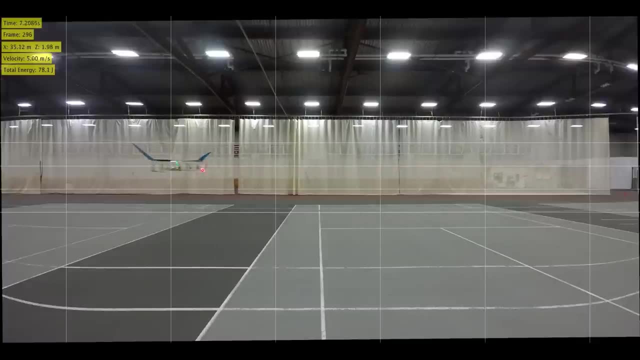 while travelling fast enough to achieve flight. Not an easy task, and the fact MIT have managed it is mind blowing. Let's see how they did it. They first needed to optimise their plane design for the application: reducing weight to minimise the energy required to maintain height and 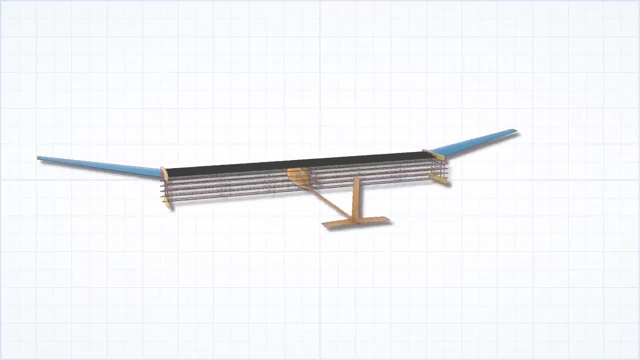 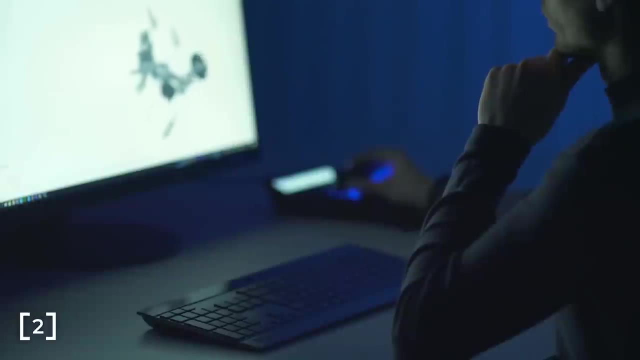 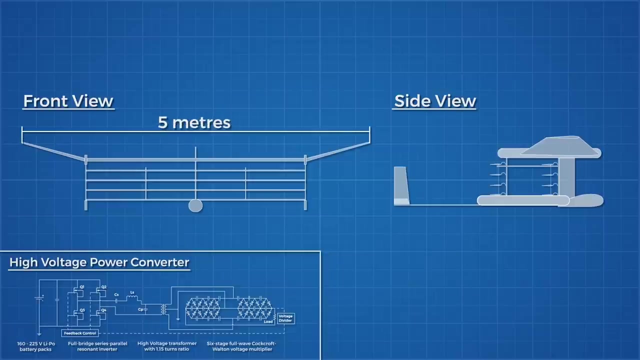 minimising drag to reduce any energy losses to the air. They did this using something called Geometric Programming Optimisation, which allows designers to specify constraints and design criteria to a program which will then find the optimal design After running multiple computer simulations. they settled on a plane with a 5 meter wingspan and a weight of 2.56 kilograms. It would require a 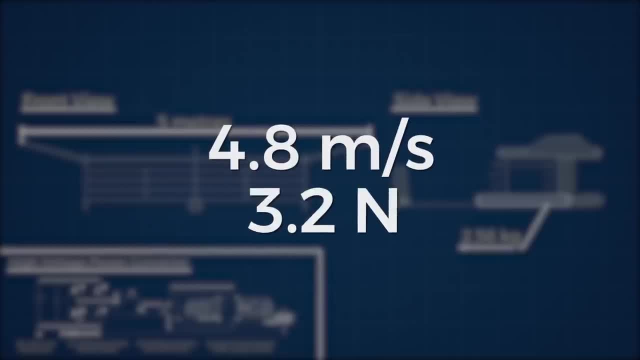 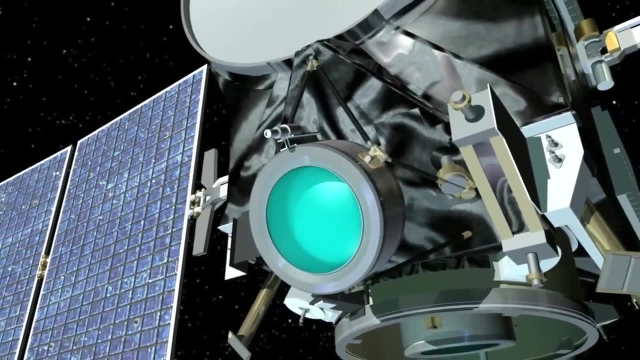 flight speed of 4.8 meters per second with a thrust of 3.2 Newtons. 3.2 Newtons is vastly more than anything achieved by the Enster or Next engines, but they don't work in entirely the same way, Ion. 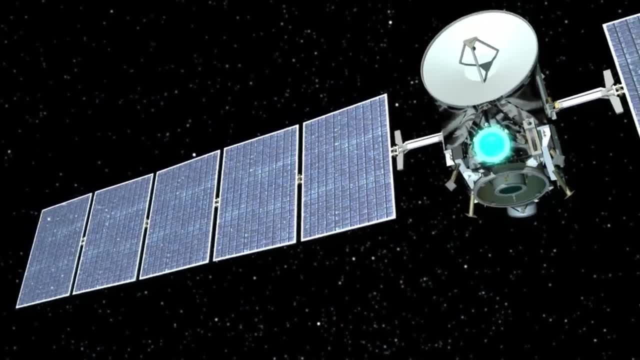 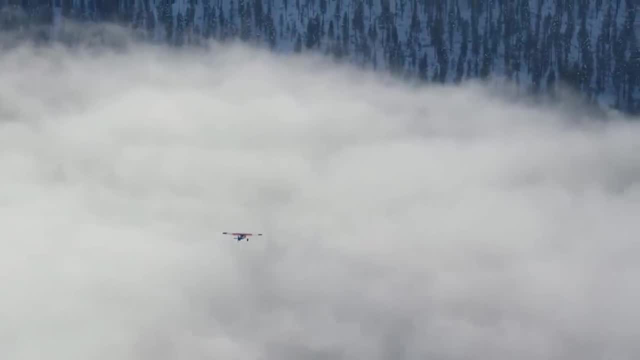 Drives for space need to carry atoms to be bombarded. Within Earth's atmosphere. there is no shortage of atoms to ionise and accelerate, and this helps counteract some of the negatives of the drag they also induce. The plane's propulsion comes from an array of ion drives carried below. 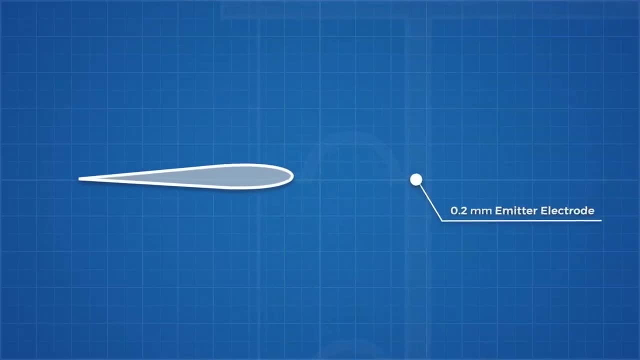 the wing, The positive anode was a thin steel wire, which helped minimise the drag it induced, while the cathodes were foam aerofoils covered in thin aluminium, These being light and capable of producing lift to offset their thrust. They were also capable of producing lift to offset their 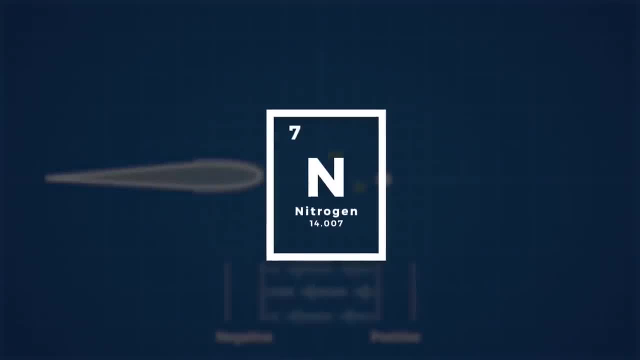 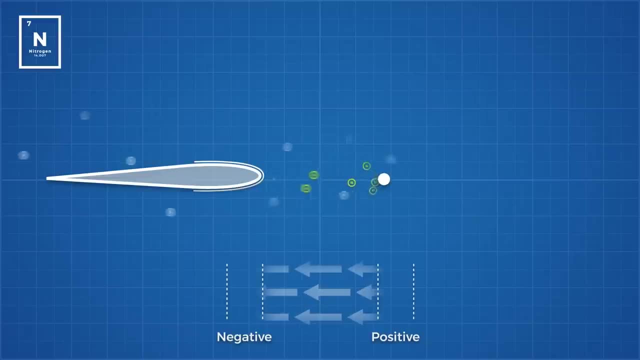 weight, In this case nitrogen, is ionised and attracted across the electric field, induced by the 20,000 volts of electric potential between them. The nitrogen ions collide with neutral air molecules along the way to provide additional thrust, creating something called ionic wind. 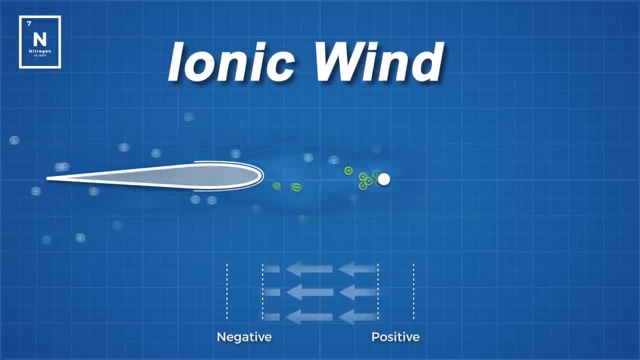 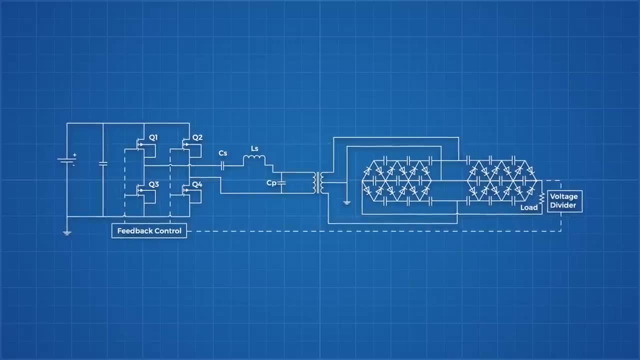 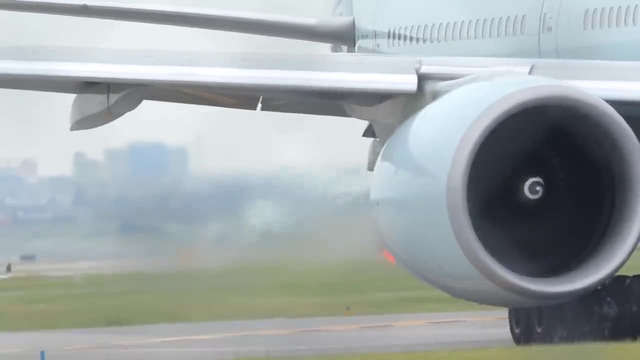 Getting that 20,000 volts of alternating current is really the most difficult part, and the team had to design their own lightweight high power voltage converter to step up the 200 volts of direct current drawn from the lithium polymer battery. This energy storage conundrum, as explained in my electric planes video. 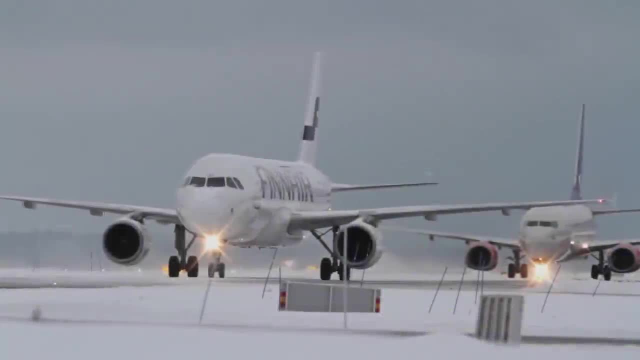 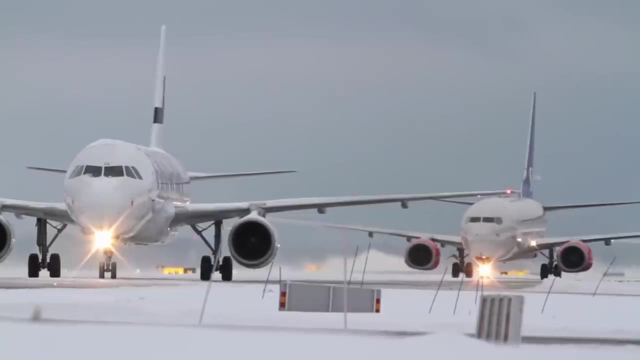 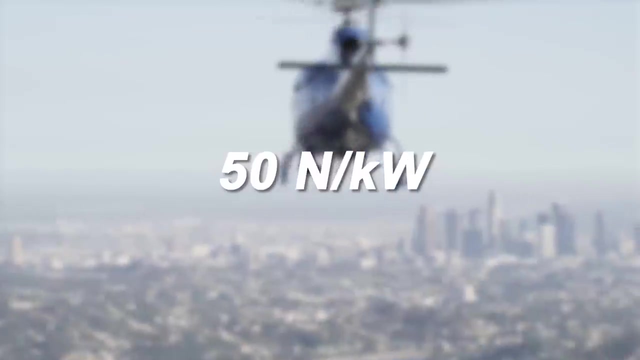 is the biggest challenge facing any technology like this. So how does this compare to conventional propulsion methods? regarding thrust to power ratios, A typical jet engine achieves a thrust to power ratio of 3 newtons per kilowatt, while helicopter rotors achieve a power to thrust ratio of about 50 newtons per kilowatt. 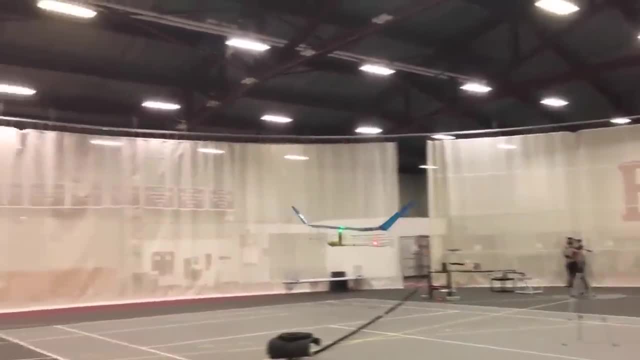 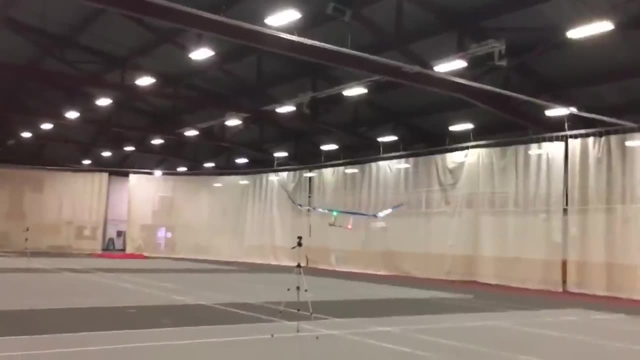 This ion propelled plane is estimated to have achieved a thrust to power ratio of 6.25 newtons per kilowatt. This means that the thrust to power ratio of the jet engine is about 3 newtons per kilowatt. So if we could find a way of powering these devices that didn't require heavy batteries. 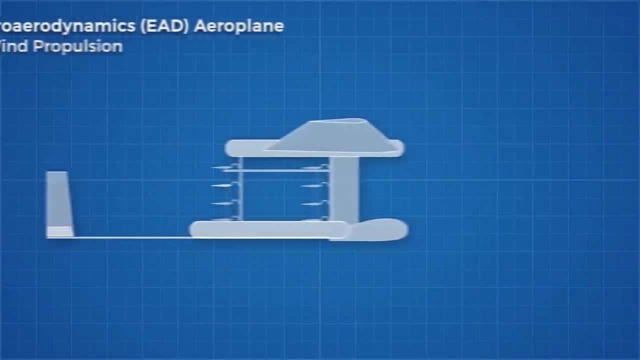 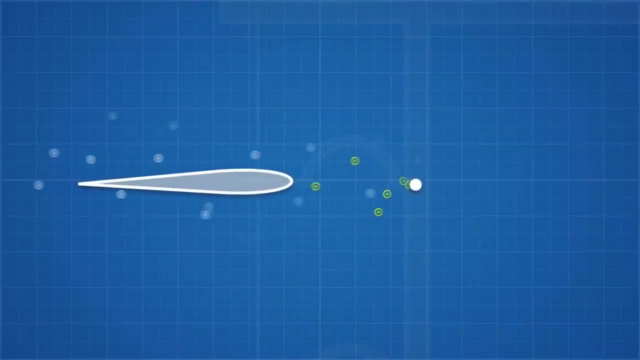 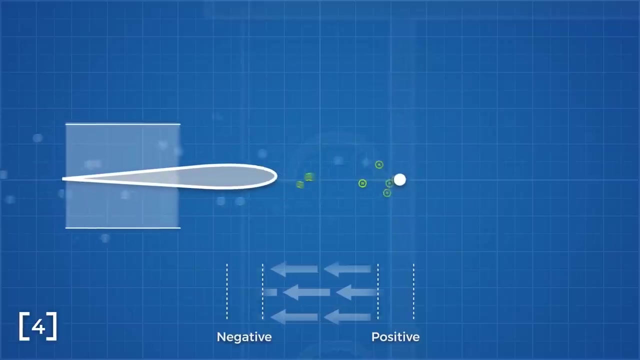 could these iron propulsion engines be used? Scaling these propulsion methods is not easy and individual electrode pairs have their limit in the current. they can pass between them via ion transport due to limits in voltage and choked flow within the electric field, just as air can become choked within a constricted pipe. 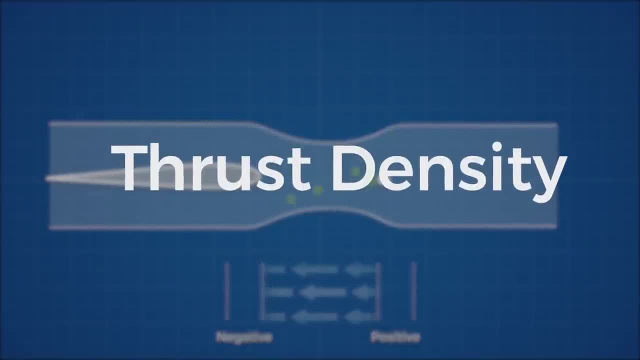 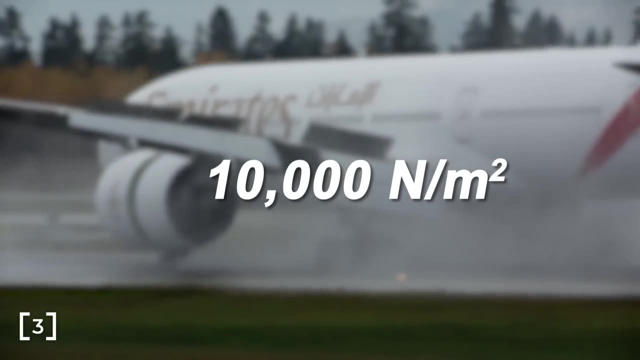 This affects something called the thrust density, which is the area over which the thrust is applied. Jet engines have a very high thrust density at over 10,000 newtons per meter squared, so we can produce a great amount of force with relatively low area. This plane achieved 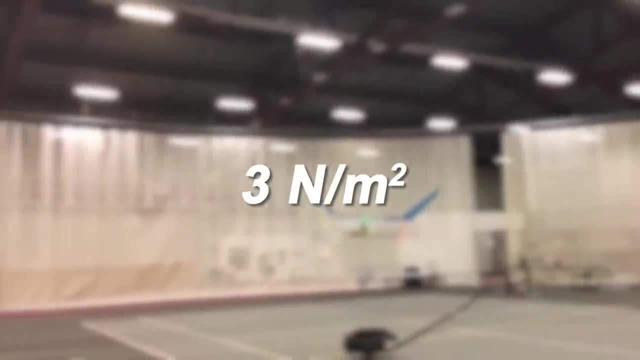 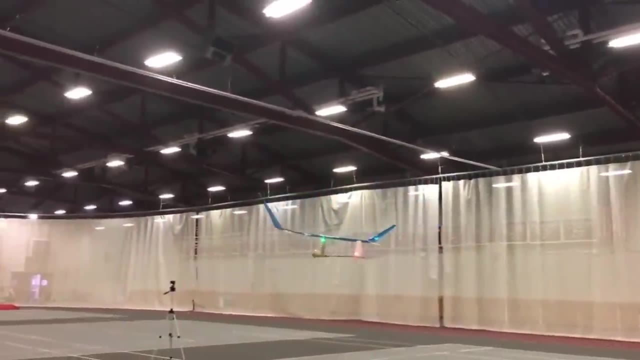 a thrust density of 3 newtons per meter squared, so it is generating very little force over a very large area. We can just about manage to provide enough force with 4 racks and 2 rows of these electrodes hanging far below the wing for a plane this light and slow. 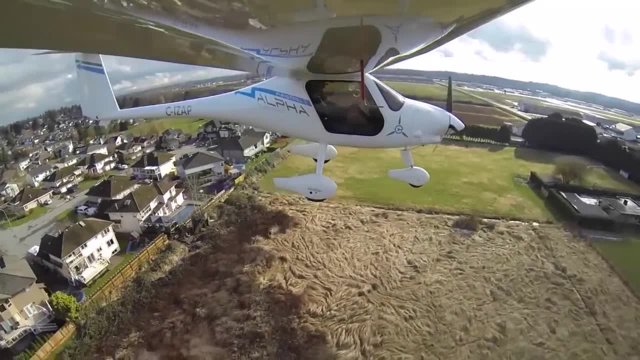 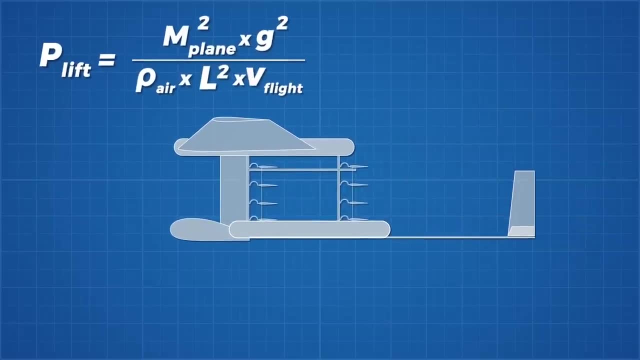 The issue here is the same issue that prevents batteries from being a viable solution. solution for planes. Power requirements do not scale linearly with the mass of the plane. they increase with the square of the mass, while the power requirements to overcome drag increase with the cube of the velocity. 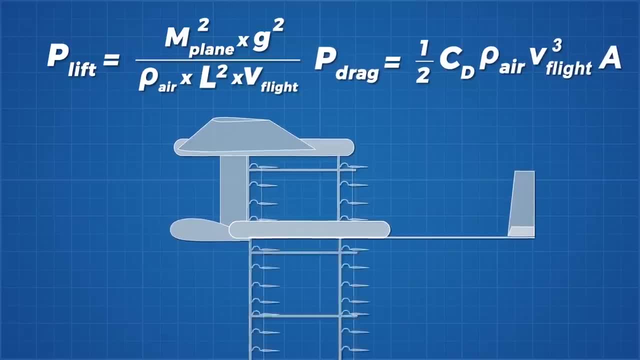 So our iron propulsion power will need to scale with it. but we cannot simply hang racks and racks of these electrodes beneath our plane. They, along with the structures required to support them, would cause far too much drag and in turn, flight surfaces would need. 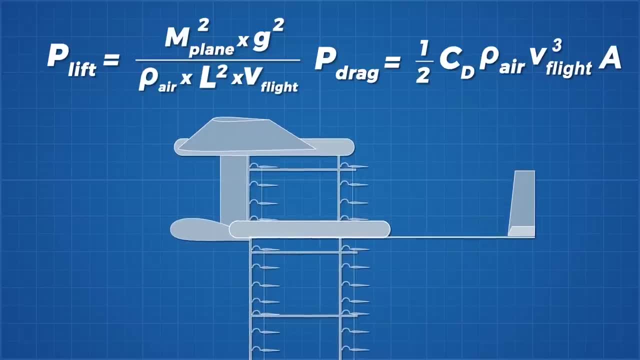 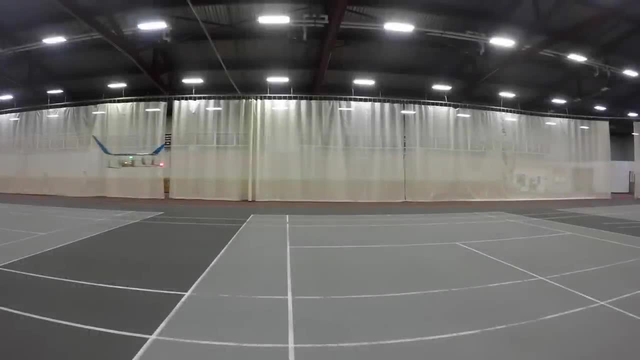 to scale to counteract the pitching moment. this would cause causing even more drag. This technology is still in its infancy and there are engineers far more intelligent than I working to figure out ways to apply it. But just think that 114 years ago, the